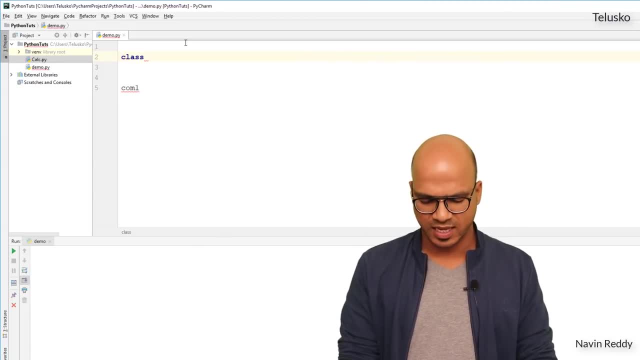 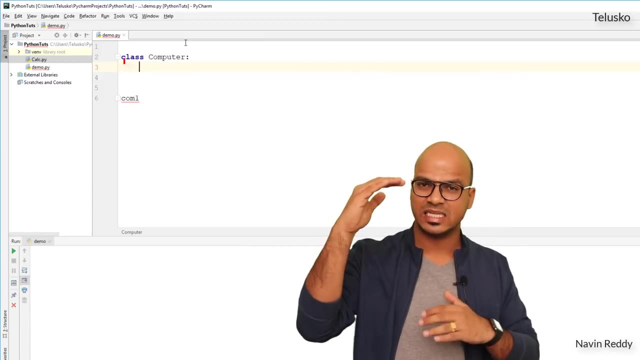 So we have to say class, and this class will of course, have a name. In this case, I will use a name as computer. Okay, now, this is how you define a class. You have to specify a colon Now after colon. this is your suite, right? 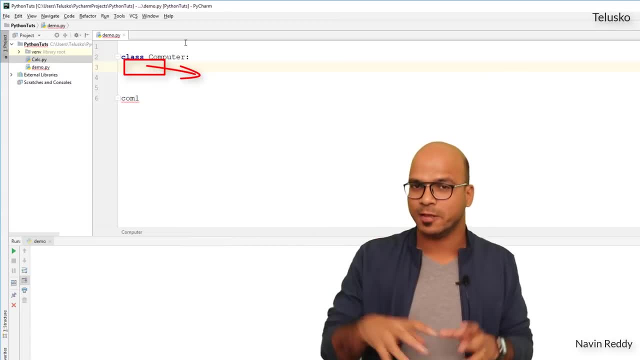 So this is where you will mention your stuff. Now, what stuff we can put in a class? Two things: The first thing is the attributes, The second one is the behavior. Oh, now, when you say attribute, it is your variables. okay, the way you create variables. 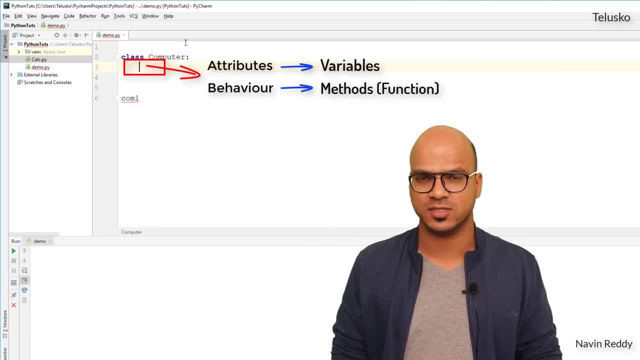 And the next thing we'll be having here is behavior, which is methods. What is methods? Functions? So now the functions which we are using from a long time, but here we call them as methods. So next time, when you are calling a function, but that function is a part of a class instead, 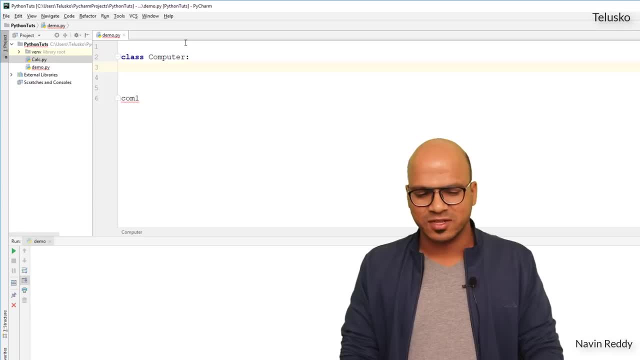 of calling them as functions, you have to say methods, right? Okay, now let's define some methods here. Now what method I'm talking about? if I say let me get a method here, we'll say def. I will say config, because every machine has a configuration right. 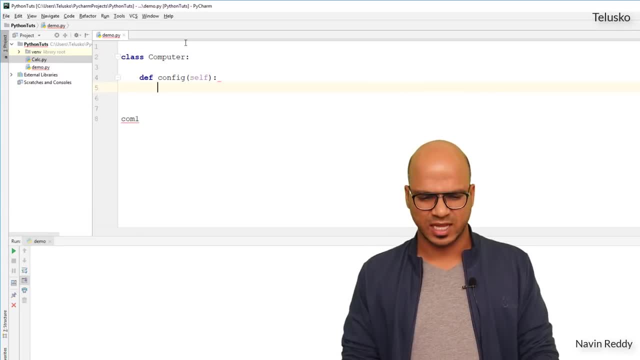 So I will say config, We got that self keyword. that That's weird. What is self? Because, see, I'm not typing it okay. So I mean, the moment I say bracket, it says self. We'll talk about that self later, but time being let's keep it there. 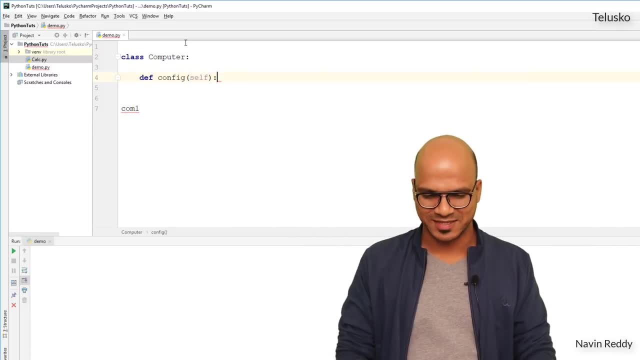 You can imagine we don't have any self here. okay, For time being. imagine we don't have anything like self, Okay, and here we'll say: we got a computer class and then we got a config method. or you can say function, but try to move from that function term to method term, right. 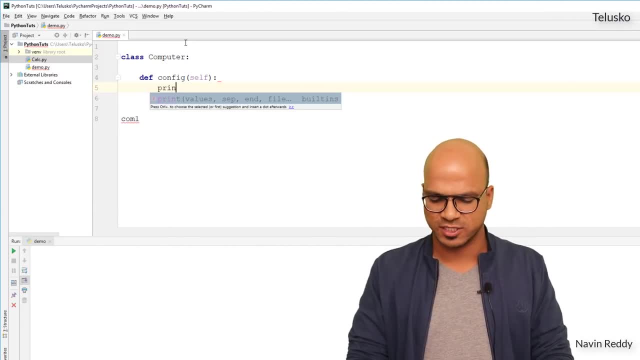 So we got a method here which is config. Here I'm printing the config of this machine and I want to say, hey, this is i5 machine with 16 GB RAM and it has one terabyte hudder. Now, this is very common config now which we find nowadays right. 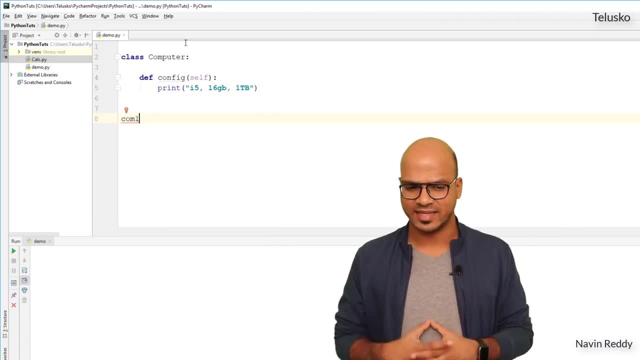 And that's what I'm doing here. So we've got a class computer, we got a method in that Example. here I'm saying: comp1 is the object of computer. but we cannot simply do that right. We cannot simply say comp1, because no one will understand what this comp1 is. 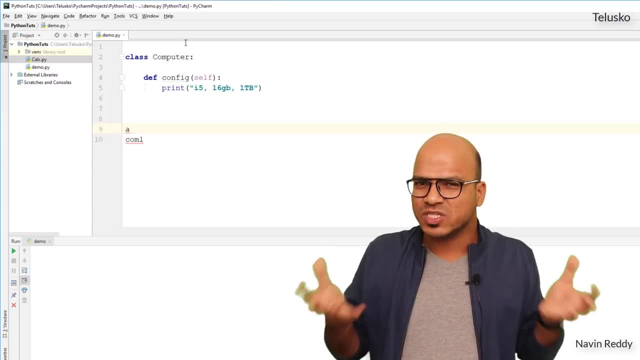 Example: if I say there's a variable a, what is a type of this variable Right Now, since in Python we don't have to statically mention the type of it? So what we can do is, when you say a equal to 5, now the type of a becomes integer, right? 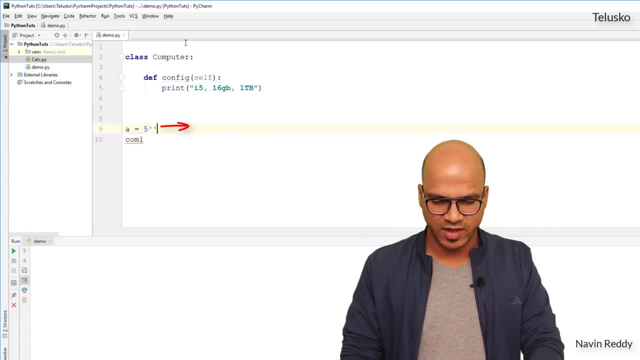 If I say a is 5.5, the type of a becomes float. If I assign a value of string type, if I say 8, even if that 8 is number- we are putting that in single code right- That becomes a string. 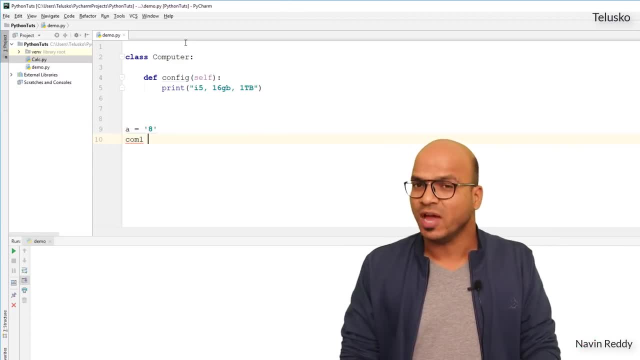 What about comp1?? Comp1 here don't have a type We have to mention. hey, this comp1 is an object of computer. In that case you will say equal to computer And you have to give this round brackets. Now, if you are coming from another, you know from different programming background like: 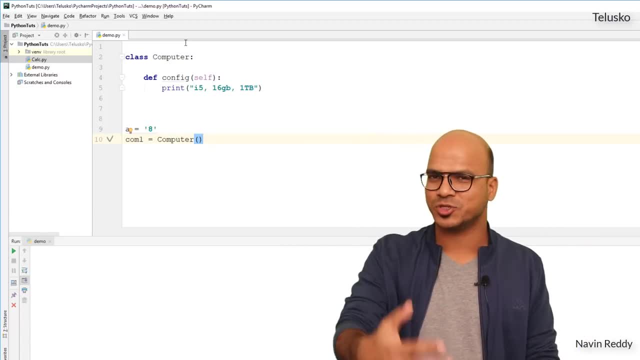 Java C sharp, we have a concept of constructor, right? So there's a constructor there. So this will give you the object of computer. Now, how do I know that? If you remember, in one of the video we have talked about a type function, right? 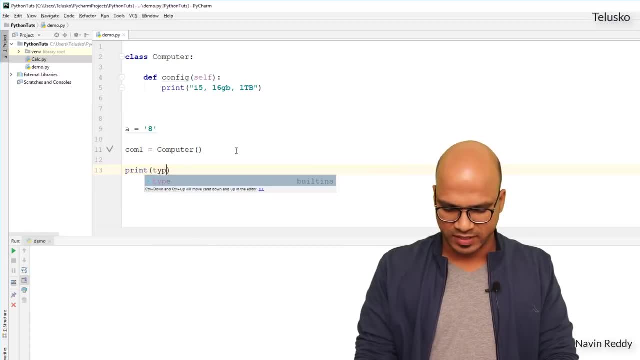 So you can use type function here. So I will say print, I will define type print, the type of comp1.. Let's see what happens, what it gives you. So if I run this code, it says, hey, this is a type of comp1. 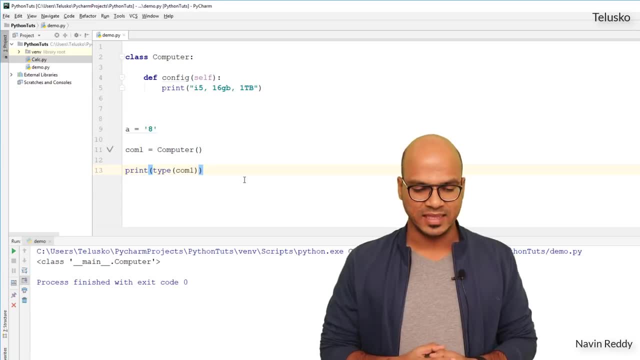 It says: hey, this is a class. Okay, Now we have a different keyword class and this belongs to a computer. That's important, Okay. So it gives you the module name. The module name is main because we are running this code from here. 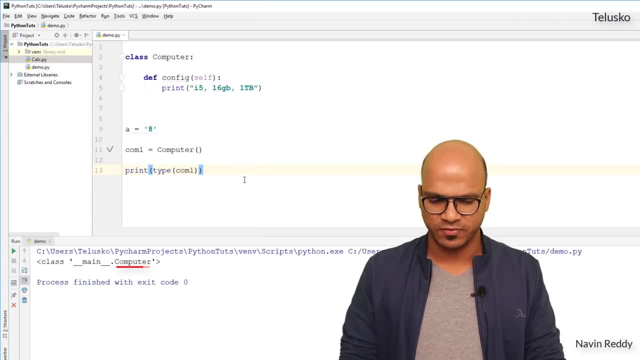 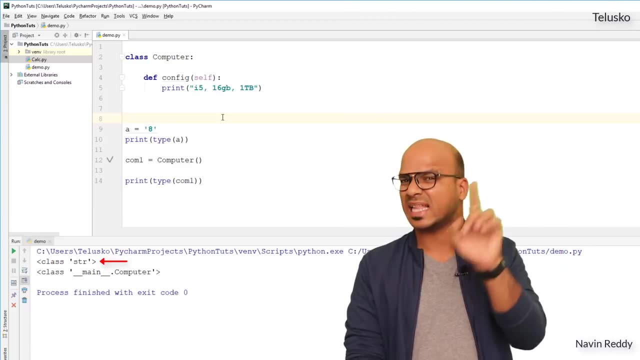 And then we have a class for this computer. Now, if you remember when we worked with string as well, string gives the same thing. So if I print the type of a, it also says the same thing. Can you see that It says class str right. 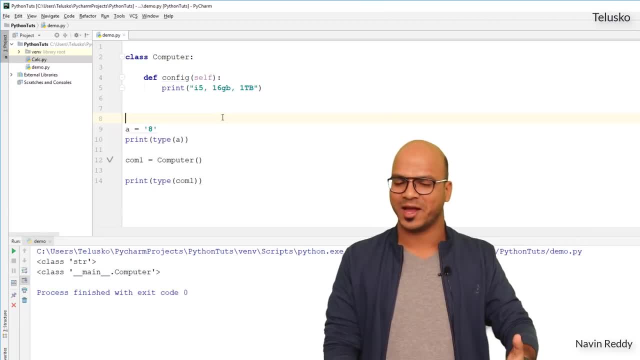 So we are using this concept from a long time, but this is where we are defining it now. So string str is also a class, The same way computer is a class. The difference is str is an inbuilt class, Computer is our class. 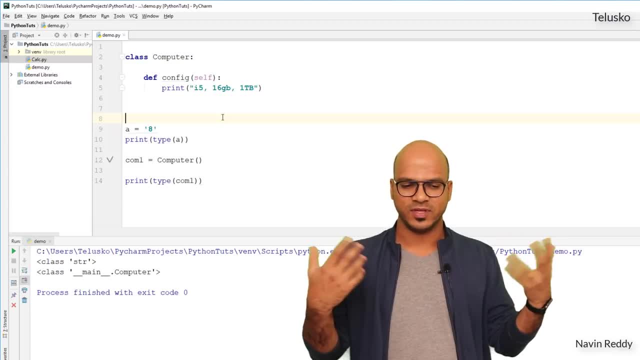 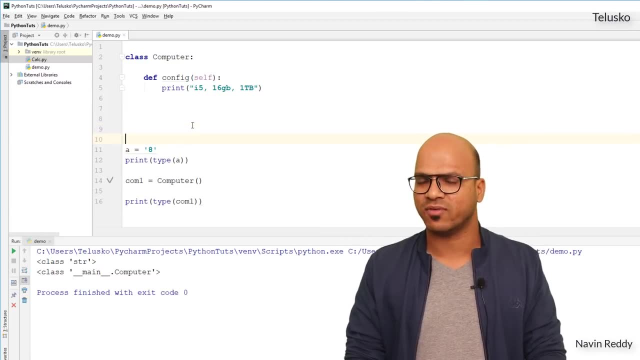 Okay, That's how you define it. So you say class computer and then we have a dev config. In fact there's one more thing: If you remember, when we worked with integers, we have also said that integers are also object. 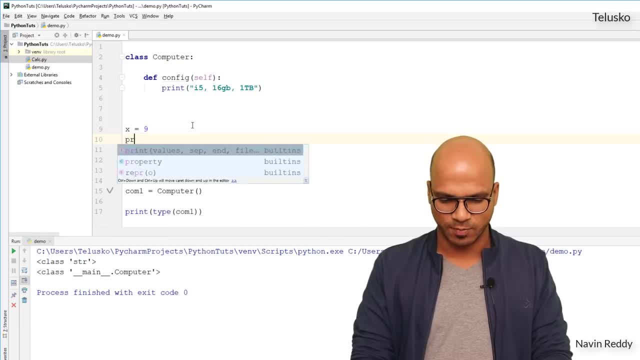 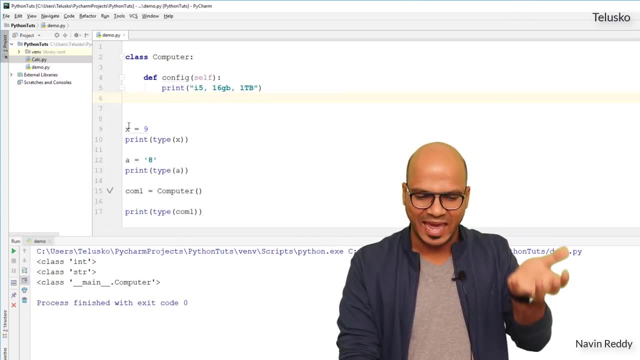 Let's try it here. I will say x equal to nine and let me print the type of x. Can you see that When I print the type of x it says class int. So even this integer, this x, is an object. 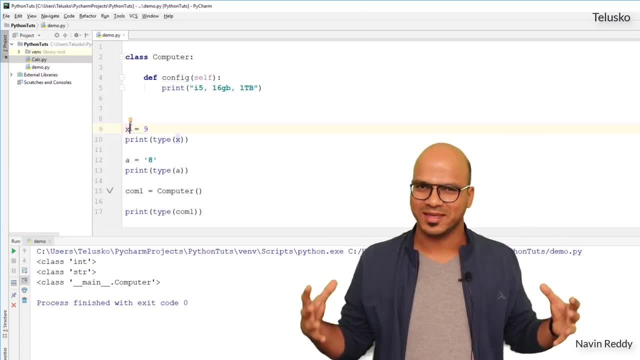 Okay, It's an object of integer now. right, So everything is object in Python, right? So there are some inbuilt objects and there are some objects which we create, And the way you create your own class is by saying class computer, whatever class name. 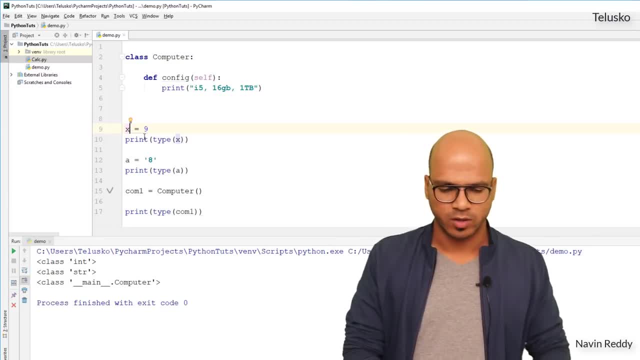 Make sure that you don't use inbuilt class name, because it will give you error, right, Or maybe you might face some bugs. So we have a. so in a class we are defining a function config and then, oh, not function method config, and then we are printing just a statement. 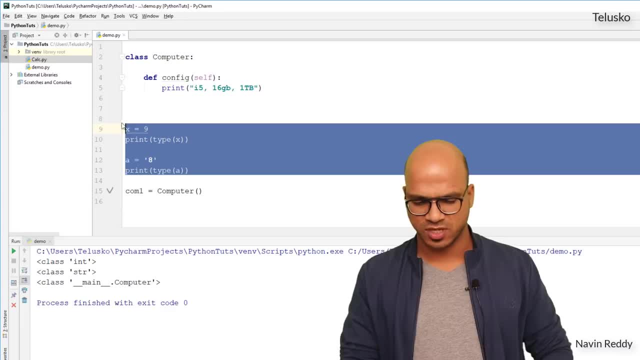 Now question arise: how will you call it? So let me remove this, all this extra stuff which we are doing. So we've got a class, we've got the object. I want to call that config. Now, what do you think? 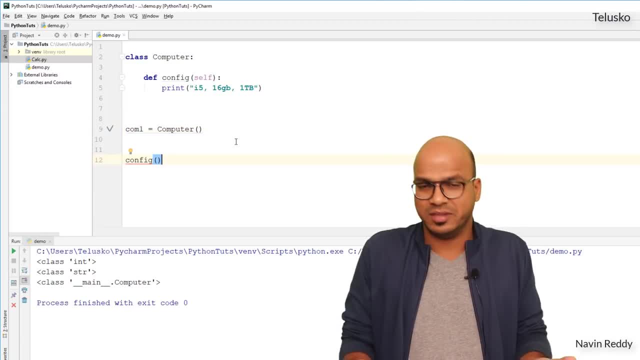 How will you do it? So normally, when you have a function, you mention the function name right here in this case, which is config, But you are getting an error. Why error? So if I go back here, it says unresolved reference, or that's weird. 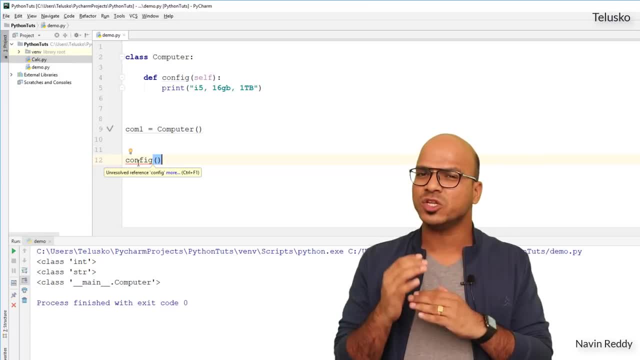 What is giving you unresolved? Because, of course, normally till this point we were mentioning the function as it is, right open. But now we have written that function or a method inside a class, So in order to access that, we have to mention the class name. 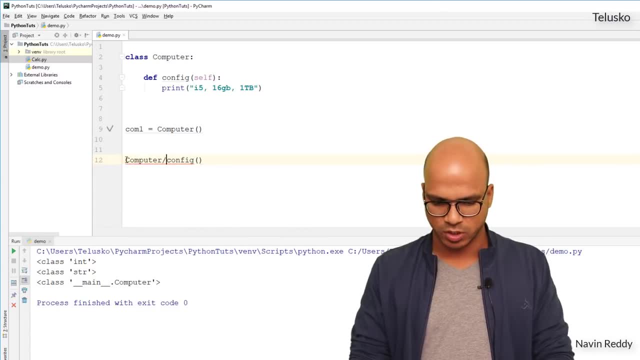 And the class name here is computer. So we have to say computerconfig, important. So steps, remember the steps. You have to mention the computer class, which is class name, and then you have to say config. So let me repeat: 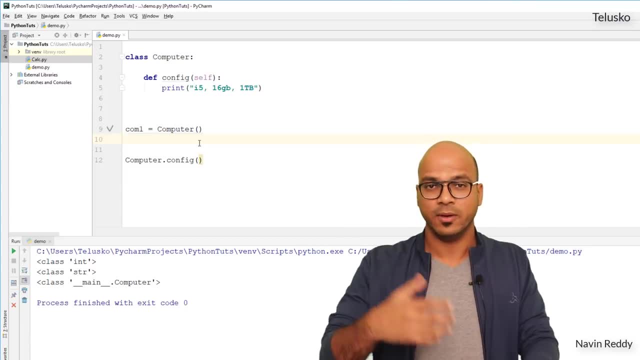 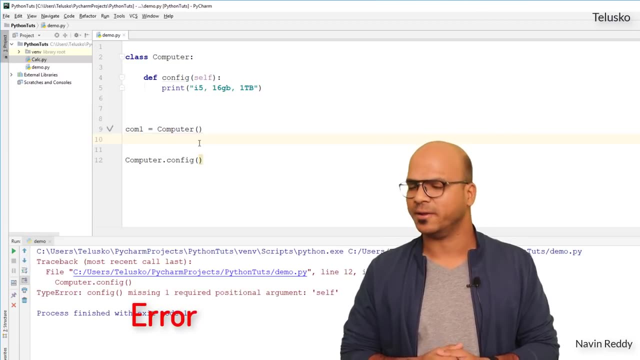 If you want to use a method, we have to mention a class name first, which is- I mean it belongs to computer, and then you have to mention config. And if I run this code, oh, we got an error, But why? 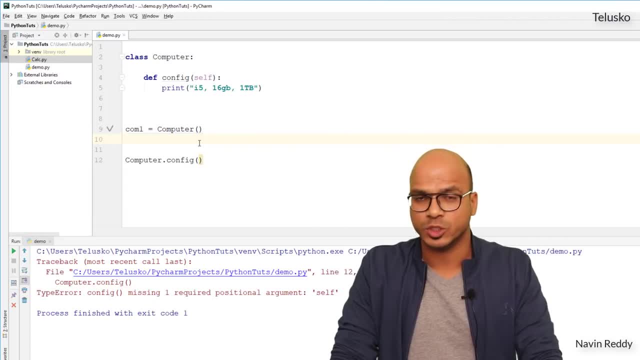 So think about this: One class can have multiple objects, right? One object, two object, five objects, maybe billions of objects, right? In this case, we are using only one object, which is comp1.. The thing is this config function or a method will change its behavior based on the object. 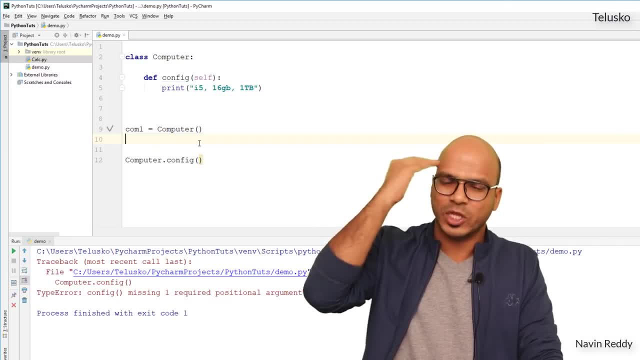 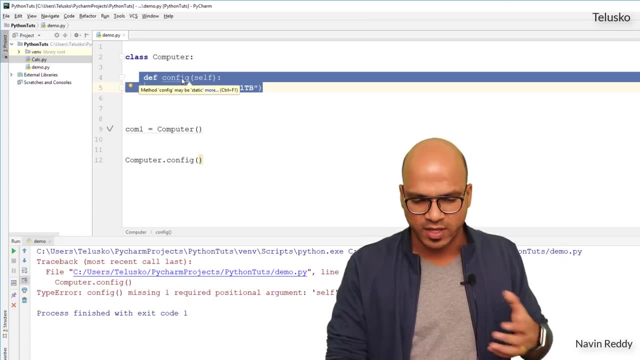 right, Because different objects have a different behavior, because, depending upon what they know, they have a different behavior. See, in this case I'm not depending on any data, right, But maybe there's a chance that this config will depend upon some data and every object. 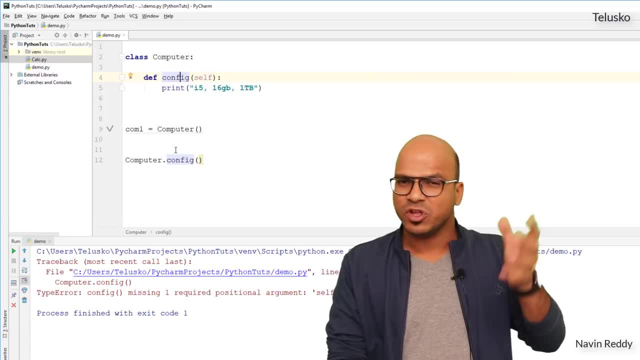 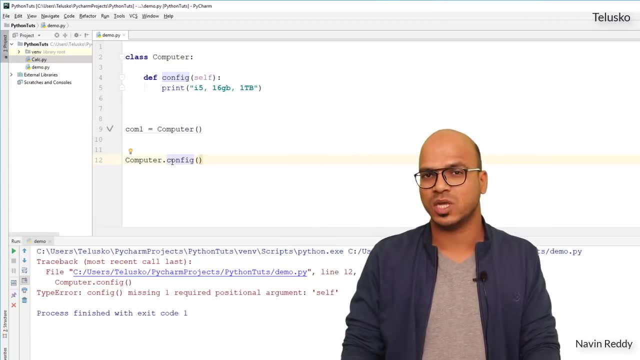 will have its own data, Right Again, we'll talk about that later. But every object is different, right? If I'm calling config, for which object I'm doing that. So if I say, hey, walk, but who am I'm supposed to say walk? 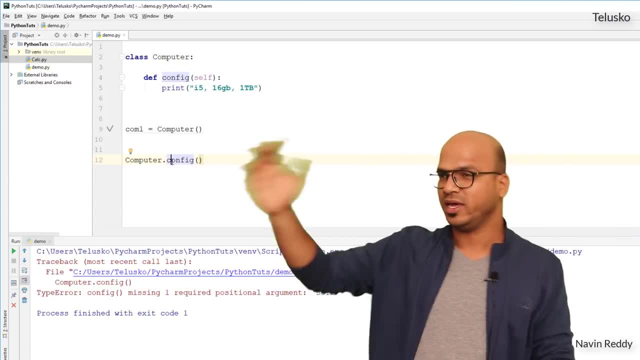 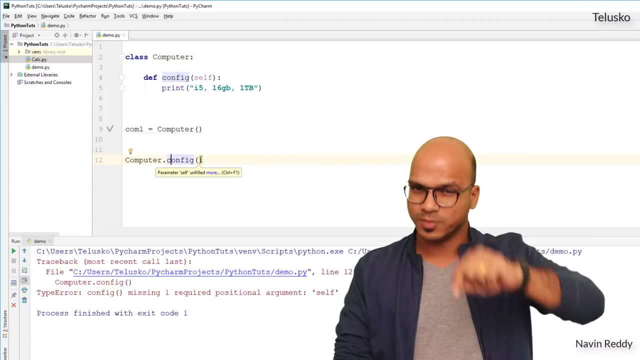 So I have to mention: hey Ravi walk, hey Mukesh walk, hey Kiran walk. So I have to mention the names as well. right, In the same way, when I say computer config, you have to also mention for which object. 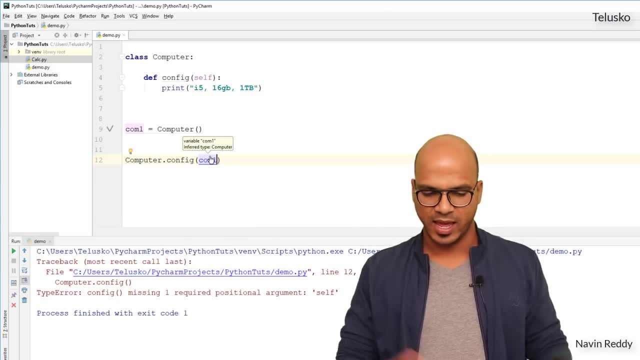 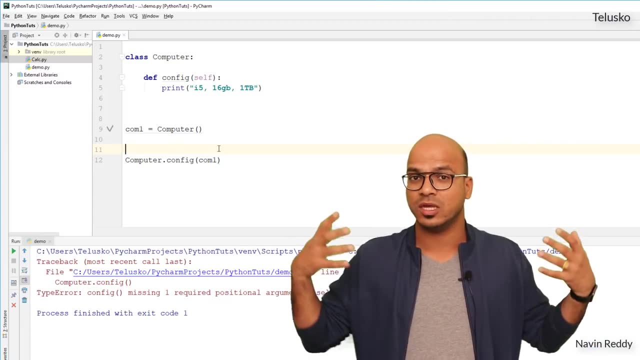 you're talking about, And I'm talking about comp1.. So I'm saying, hey, I want the config for comp1.. Now, luckily we have only one object here, so there's no confusion. But let's say, if you have thousands of objects, you have to mention the object name as well. 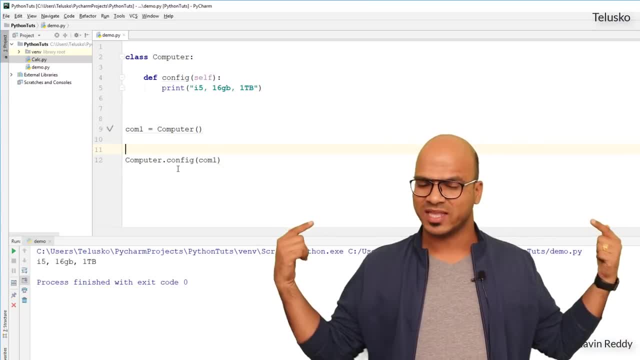 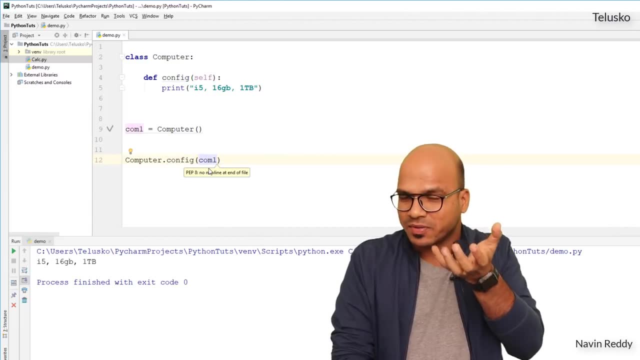 So we are doing comp1 here. So if I run this code now, oh, it works. You can see that we got the object name. Okay, We got the output. So we are calling config and we are passing comp1.. And this comp1 is a parameter, right, it's an argument. 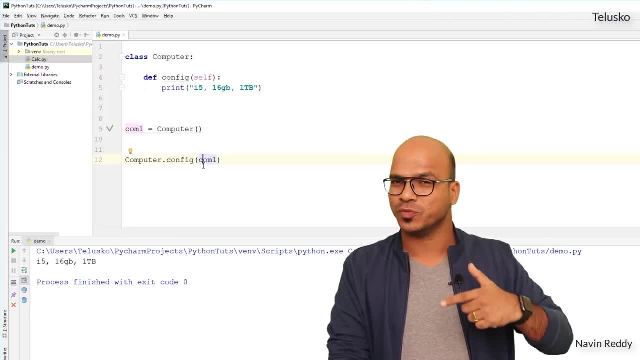 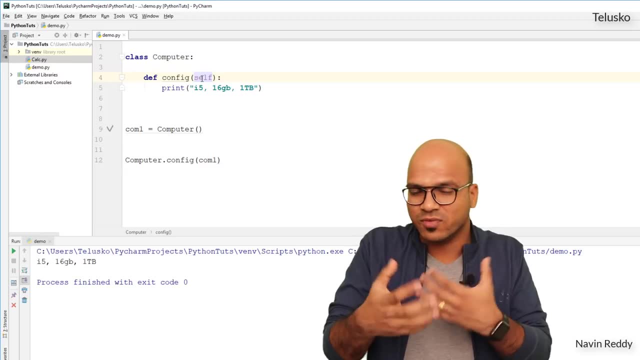 So when you call config, you're passing this comp1 as the argument and it is going in self. So what is this self? Self is the object which you're passing Again. this thing will get more clear once you see further videos, right? 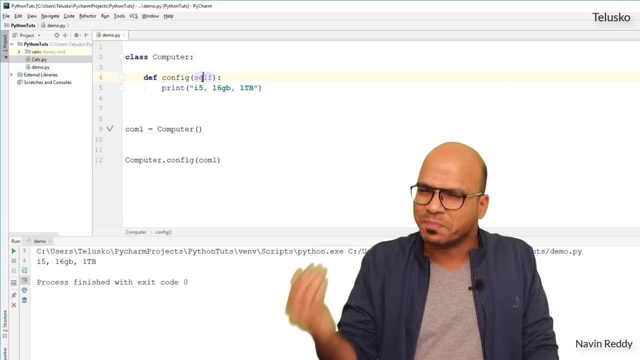 So this is a complex concept if you're learning OOPS for the first time, But step by step, everything will go inside your brain. okay, So this is the first layer. Again, in the next video, we'll talk about some more layers to it. 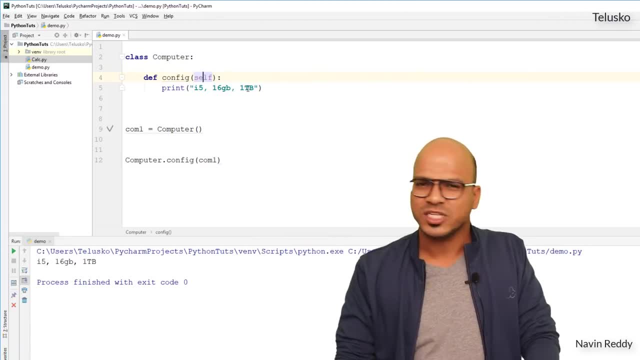 We'll add more layers and then I will make sure that you'll get everything about it. Okay, Let's create some more objects, okay? So I will say: comp2 is equal to computer, right? So we got comp1,, we got comp2.. 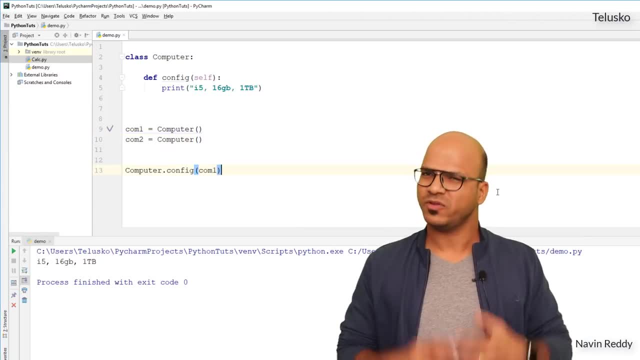 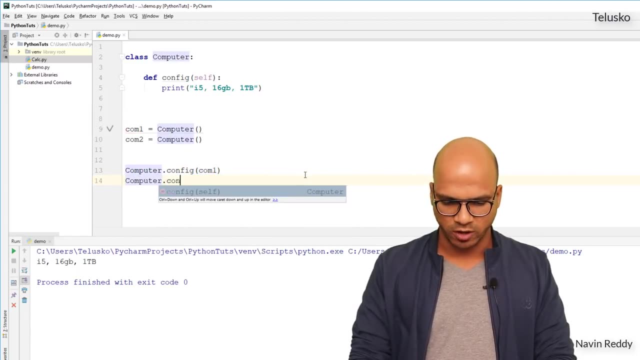 So in total we have two objects, which is comp1 and comp2, but we have only one class, which is computer. If I want to call config for comp2, what you will do, you will say computerconfig, and this time you're saying: hey, I want to call config for comp2.. 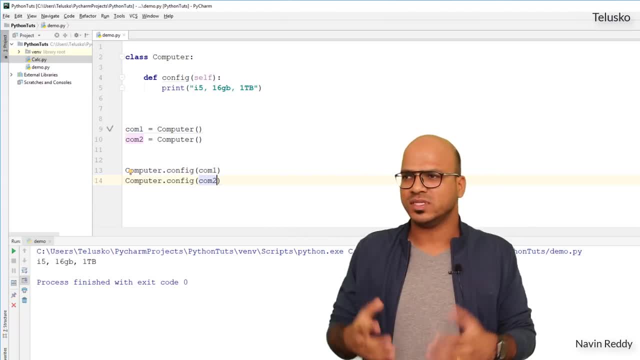 So in the first instance I'm saying, Mukesh, walk right. or I will say, hey, human walk. In black and white, In black and white, I'm passing Mukesh. I will say, hey, human walk. 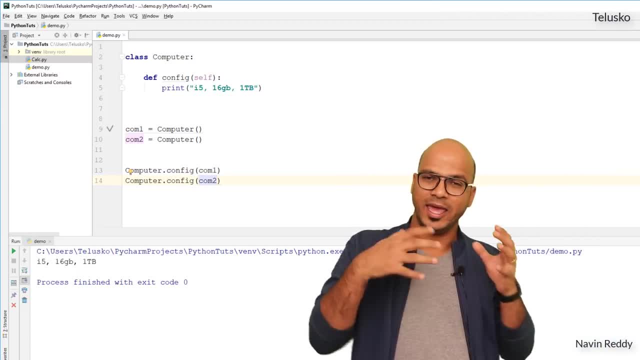 In black and white. I'm passing Ravi right In the same way. here I'm saying: hey, computer, show me your configuration, and I'm talking about comp1.. Hey, computer, I want your configuration for comp2.. 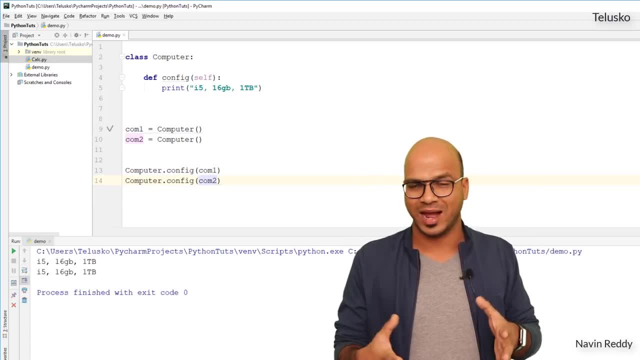 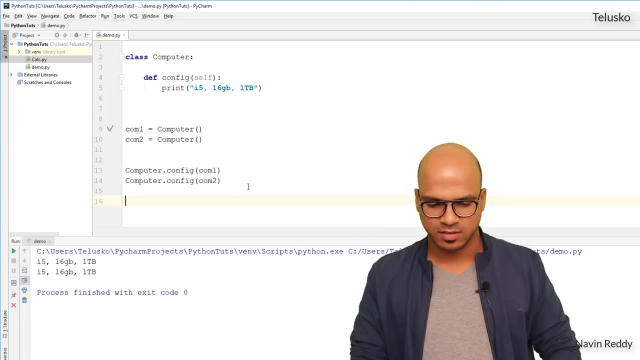 So from this code you can see we are getting same data, because at this point we are not changing data for different objects. We can do that later. So there's one way, right? If you want to call config, we have another way. 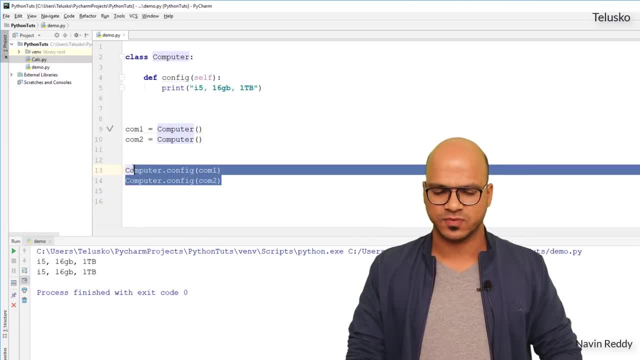 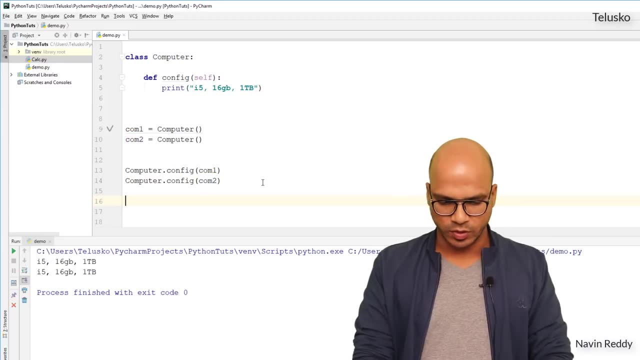 If you think about this, this looks good, right, This looks clean, because we are saying: hey, config method belongs to computer, And then we have to pass the object name, which is comp1.. But there's one more way. What you can do is you can mention comp1.config. 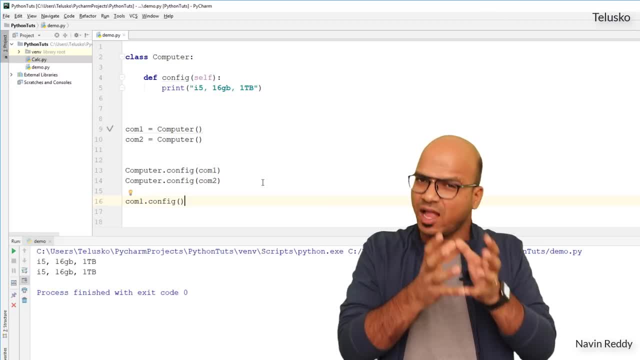 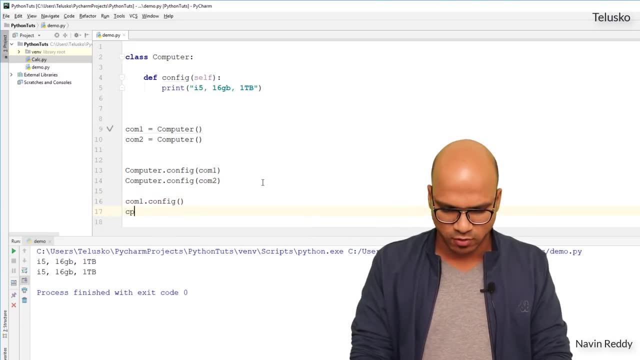 Now, in this case you are using the object itself to call the function. So you're saying comp1.config. But question is: we are not passing it right. Example: let's do it for comp2 as well. I will say comp2.config, and you can see, this time I'm not passing anything inside config.